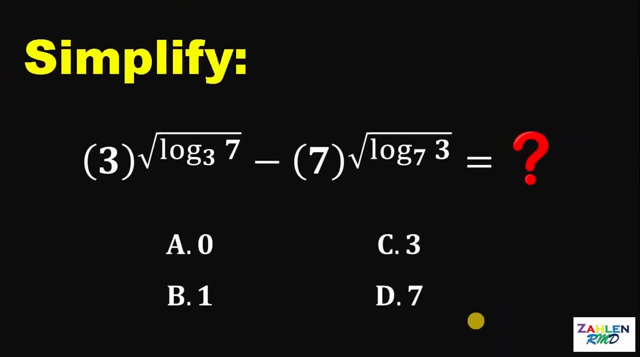 Good day everyone. Here's our math challenge for today And here's our question. Simplify 3 raised to square root of logarithm of 7 to the base of 3 minus 7 raised to square root of logarithm of 3 to the base of 7.. Now here's our choices. 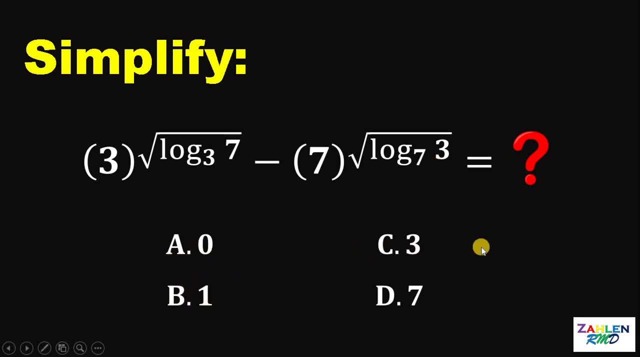 Letter a is 0,, letter b 1,, letter c 3, and letter d 7.. Now, if you want to try this problem, you can pause this video. You have 20 seconds and timer starts now Timer. 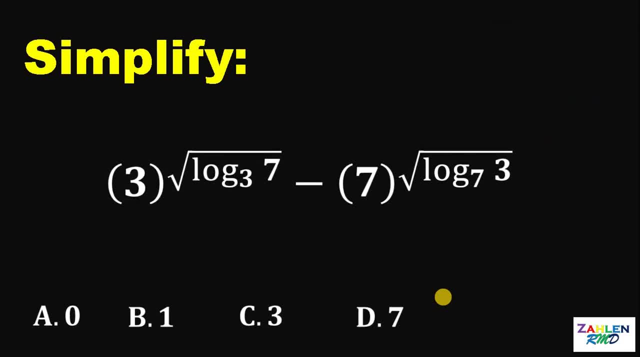 Now let's answer this question together. Our goal is to simplify this expression: 3 raised to square root of logarithm of 7 to the base of 3 minus 7 raised to square root of logarithm of 3 to the base of 7.. 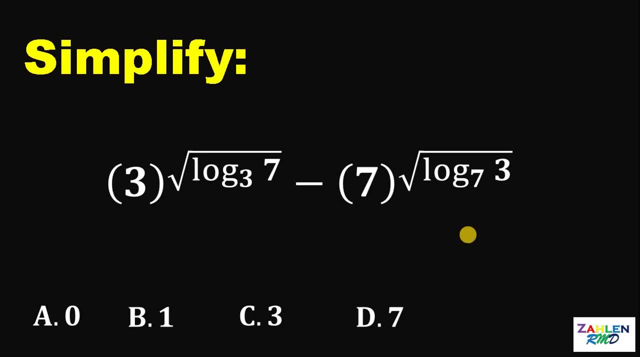 Now, how are we going to answer this question? One way to answer this question is realize that if we have logarithm of a to the base of b, it is equivalent to 1 over logarithm of b to the base of a. Therefore, this logarithm of 3 to the base of 7 can be written as 1 over logarithm of 7 to the base of 3.. 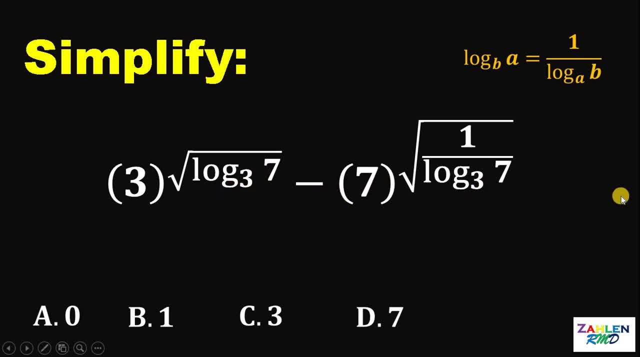 Now we have common term logarithm of 7 to the base of 3.. So we can replace this with another variable. We call this as n, So let n equals logarithm of 7 to the base of 3.. 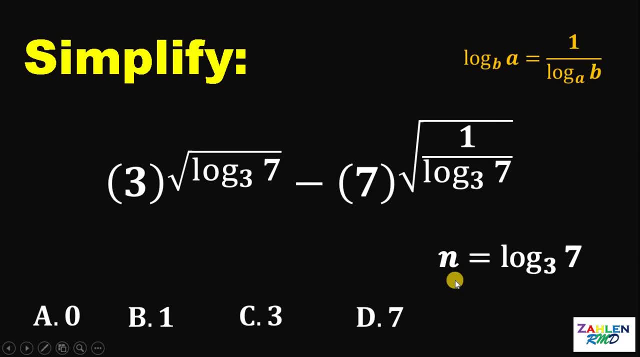 Therefore, those expressions can be replaced with variable n. Thus our expression becomes: 3 raised to square root of n, minus 7 raised to square root of 1 over n. Now, at this point, take note that if we have a logarithm equation, p equals logarithm of a to the base of b.